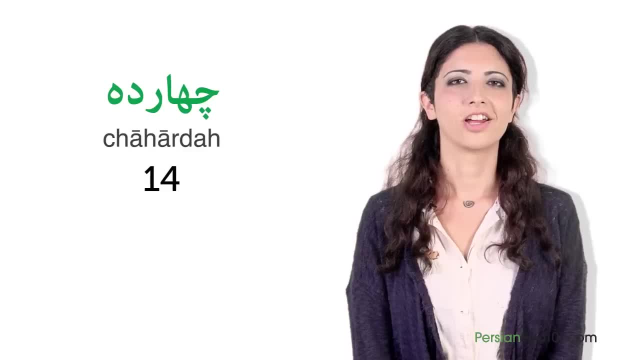 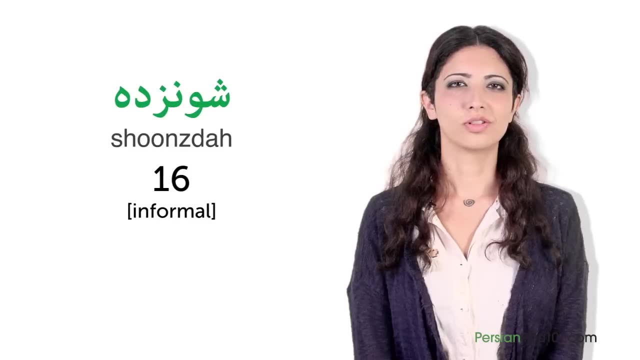 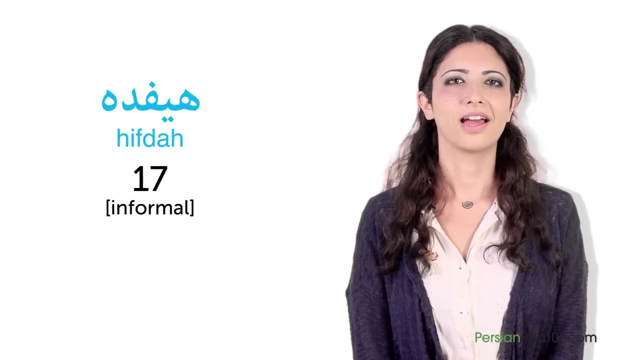 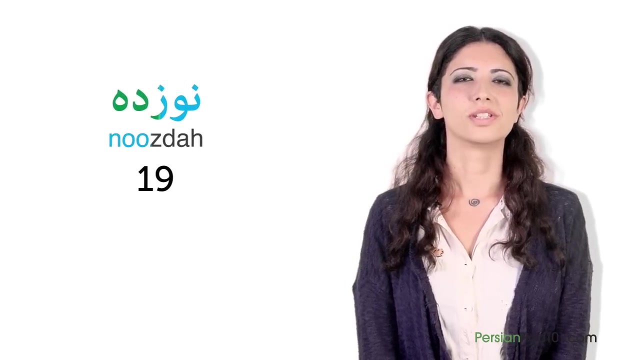 14,, 14,, 15,, 15,, 16,, 17,, 18,, 19, 20, 17,, 17,, 18,, 18,, 19,, 20 And finally we have beast Beast. 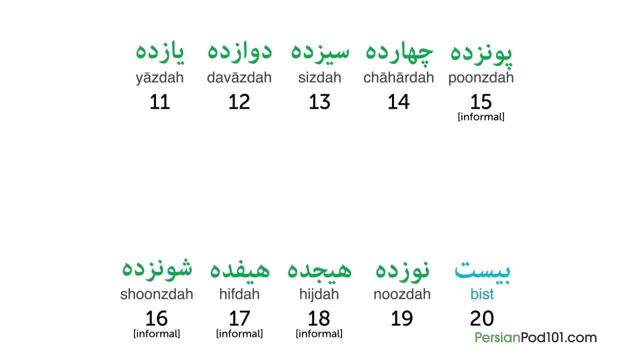 Beast. Okay, now repeat after me. I'll say the numbers and give you time to repeat each one. Yazda Davazda Sizda Çaharda Punzda Şunzda İvda İvda Hizda Nuzda. 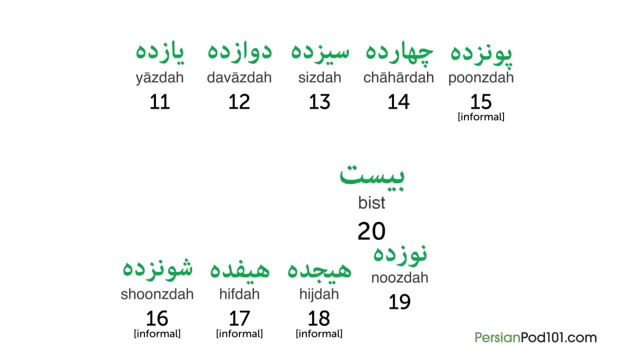 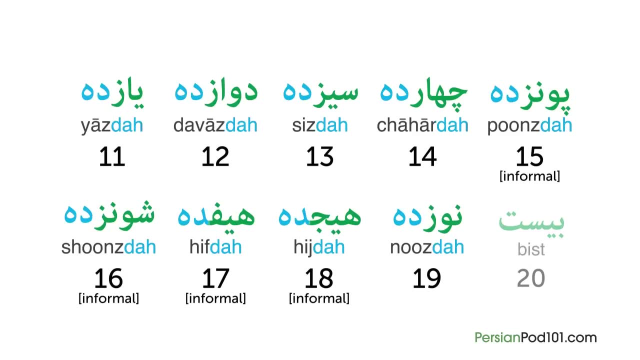 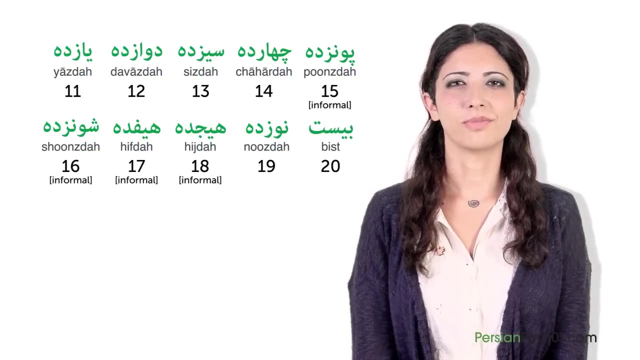 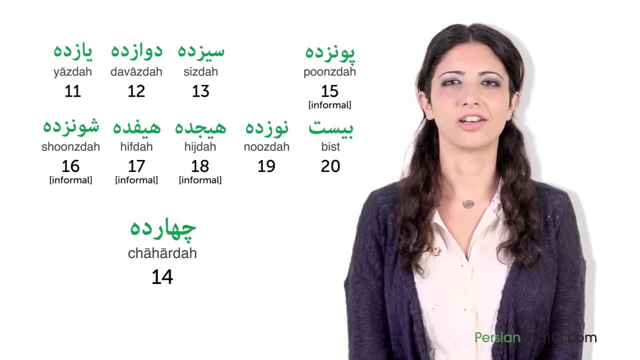 Pist. Notice that all these numbers- except 20, have dah in the end. These numbers may seem harder to remember, so you really just have to memorize them. Some of them look a lot like their base numbers, like Çarda and Çahar, but others you will. 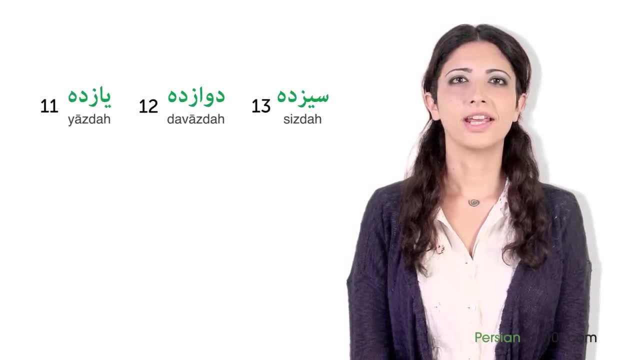 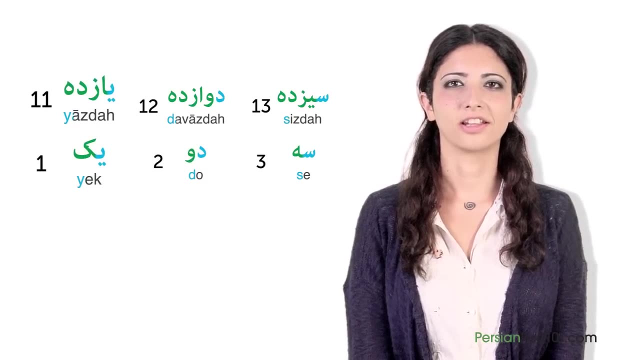 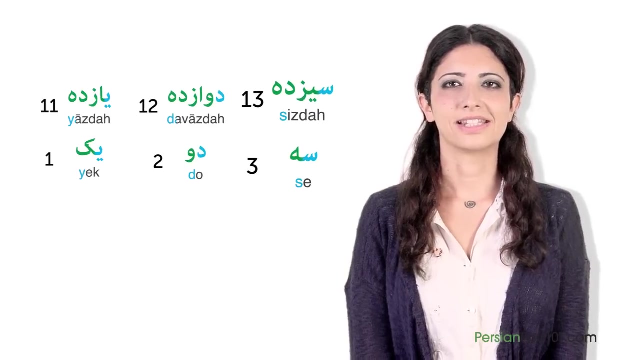 have to memorize. Luckily, you can get a hint from the similarities of their first letter to their base numbers, like Y in Yek and Yozda, D in Dor and Davozda, S in Sizda and Se and so on. 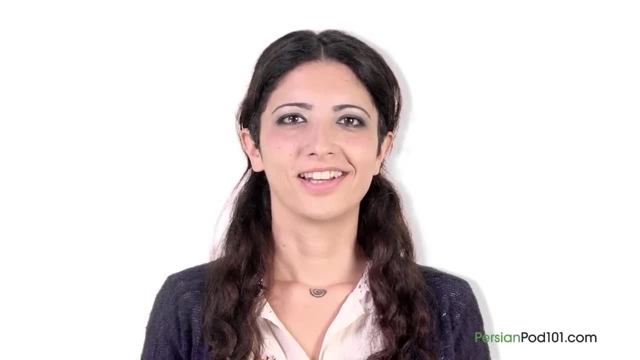 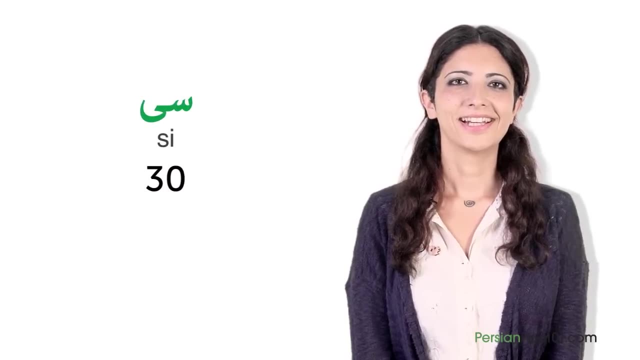 Let's not stop at 20.. Counting to 100 is super easy. Now I'll give you the tens. Si, Si, Çehel, Çehel, Çehel, Çehel, Çehel, Çehel. 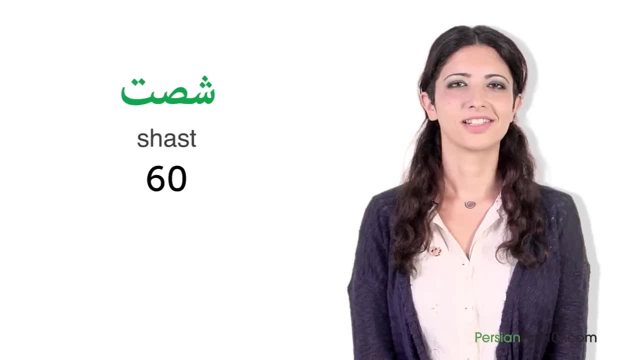 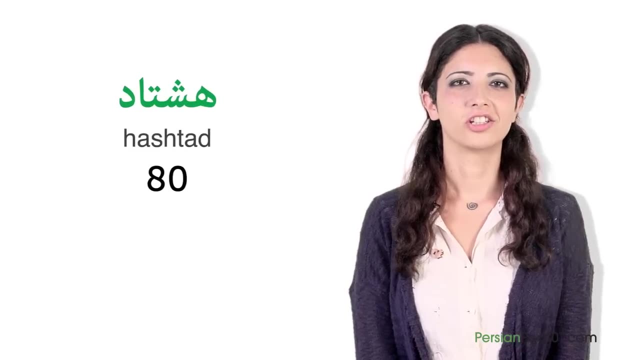 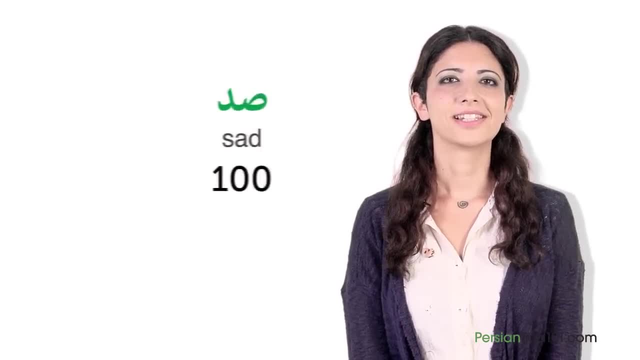 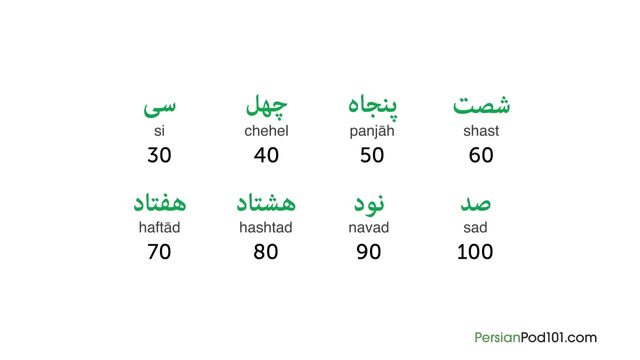 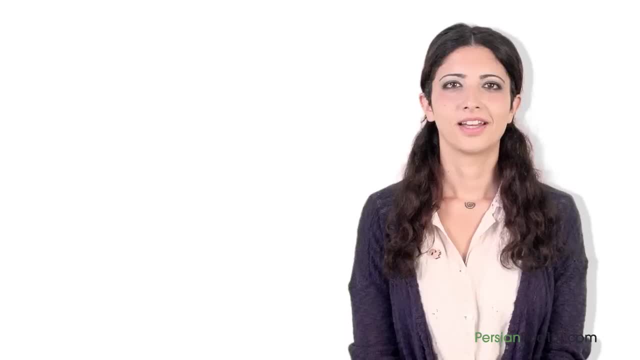 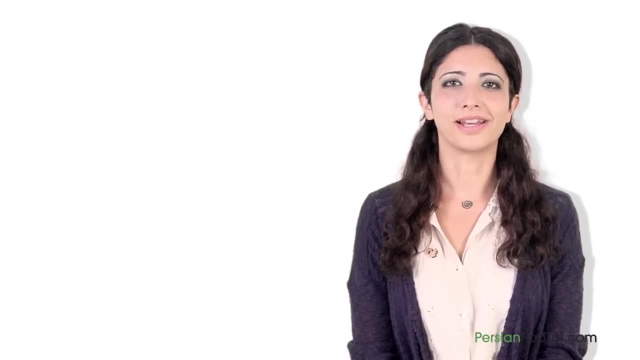 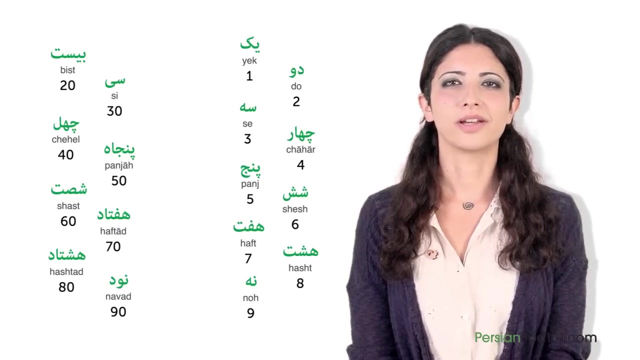 of their first letters to their base numbers. The last thing to learn today is how to form compound numbers above 20.. This is also super easy. Take the tens and add any number from 1 to 9. Then just put the particle or between. 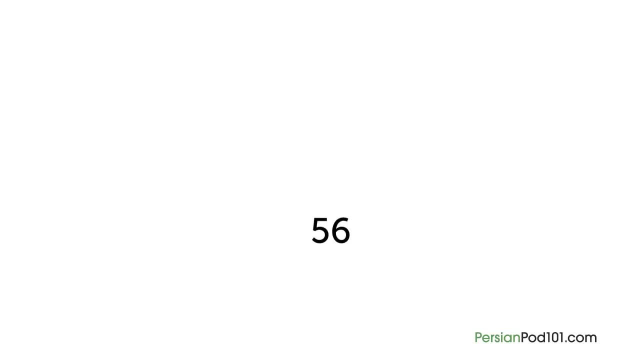 them. So how would you say 56 in Persian? Let's take it step by step: 50 is panjah, and then you add the particle, or in the middle, before adding 6, shesh, Panjoshesh, It's done. 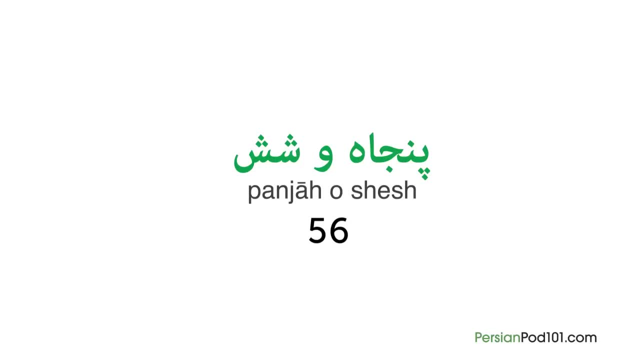 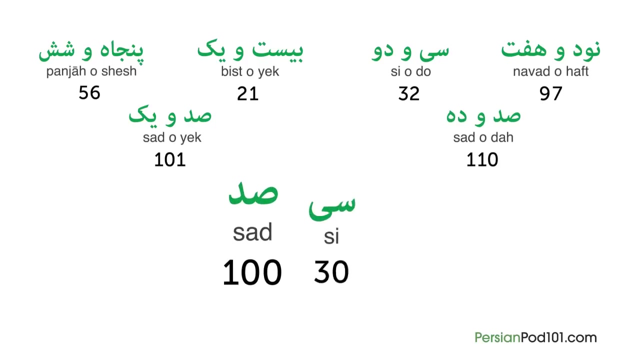 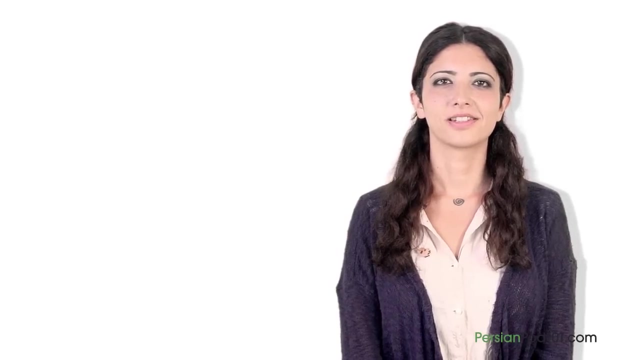 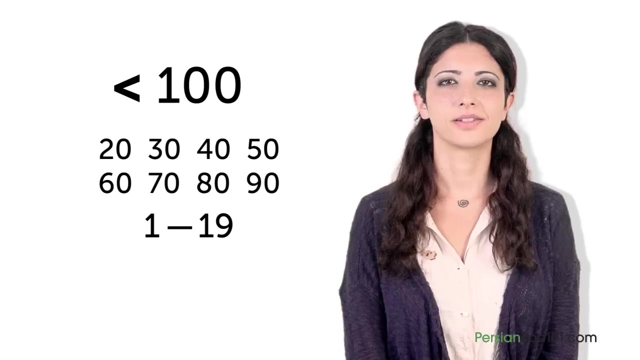 Isn't that easy. Let's make some more numbers: 21, 21, 32, 97, 101, 110, 131. Now it's time for Anita's advice For numbers up to 100, you just need to memorize 1 through 19 and all the tens, If you remember. 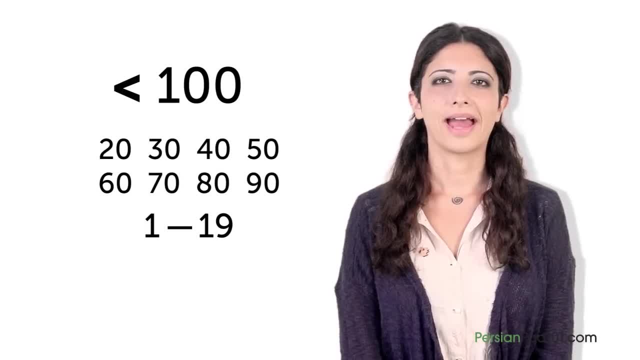 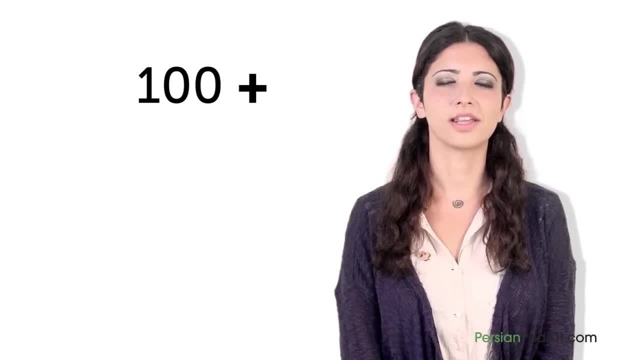 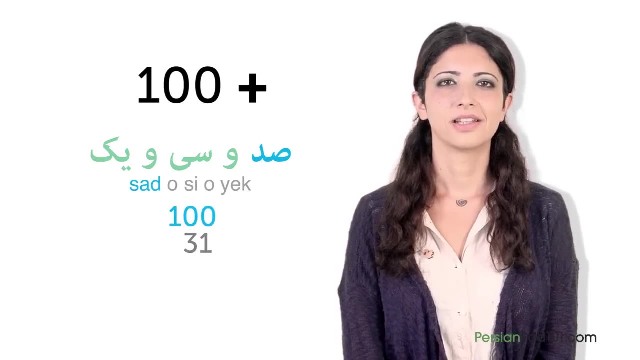 them. well then, you can easily make any number by adding an or between them, For beyond 100, it will be the same. You just need to memorize the hundreds. So when we made 131, we said hundred sadh the particle, or then 30. Then 30. When you have a number that is above 100,, 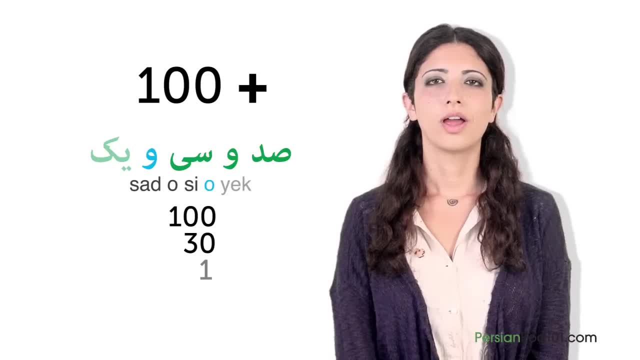 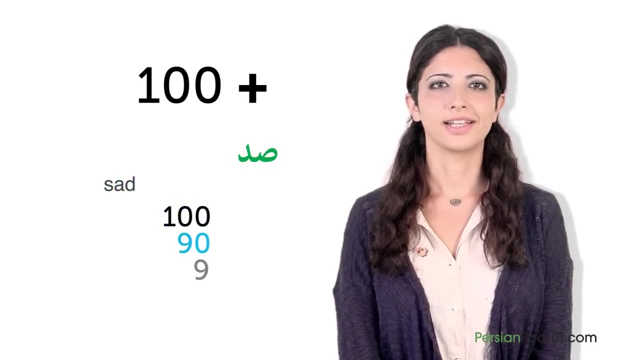 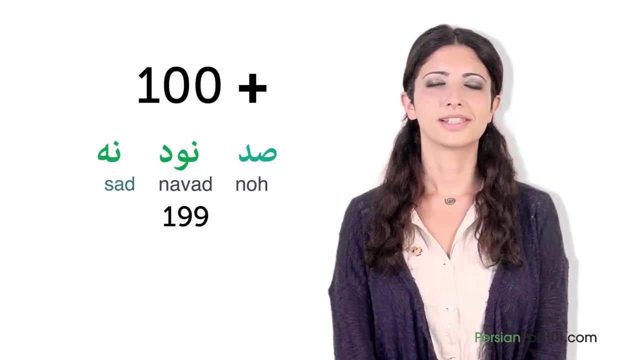 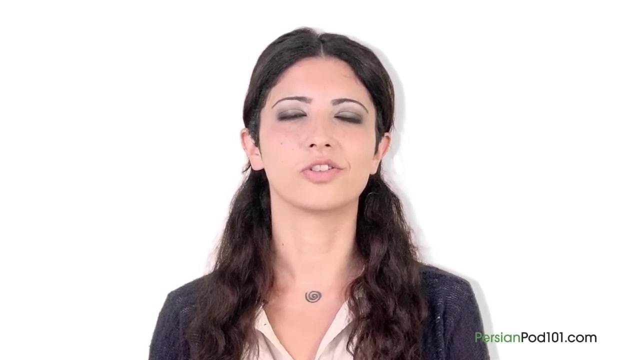 and another and finally. so what do you think? 199 is in Persian? a hundred sat ninety navad nine, no. so sado navado no. after only two lessons, you are now able to count to 199 in Persian. In the next lesson, we're going to put your number knowledge to use. 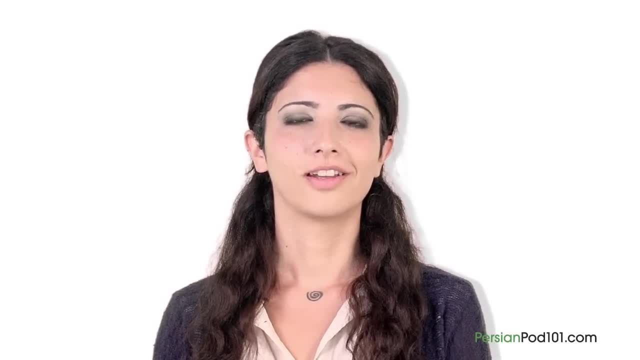 Do you have all the skills you need to go shopping in Iran? If not, I'll be waiting for you in our next Persian in 3 minutes lesson: Khuda hafiz.